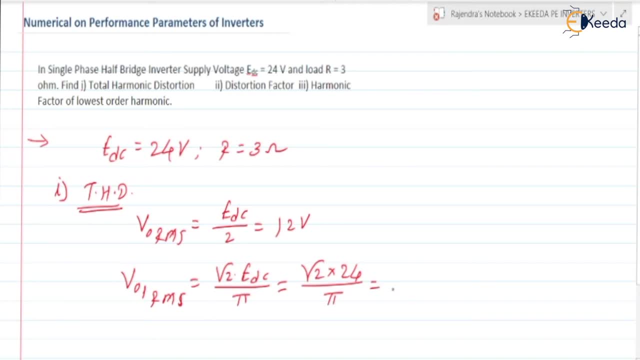 Okay. so if you check, it is equal to root 2 into 24 divided by pi, So it is 10.8.. Okay, 10.80 volt. This is a V01 RMS, Okay Next. so from this can we find THD? Yes, we can find. THD is equal to, yes, THD total. 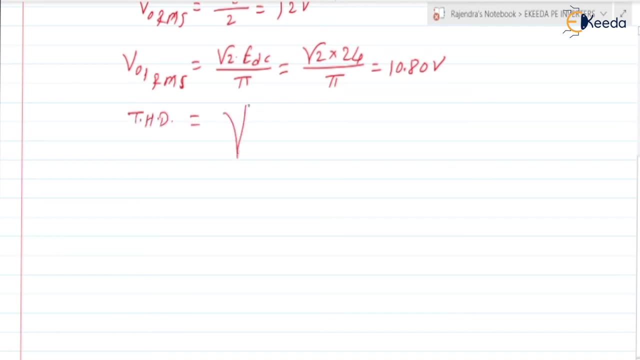 harmonic distortion is equal to under root. yes, V0 RMS. square minus V01 RMS. square divided by right: V01 RMS. Okay, So if you put the values is equal to, we will be getting under root. yes, it is a 12 square. 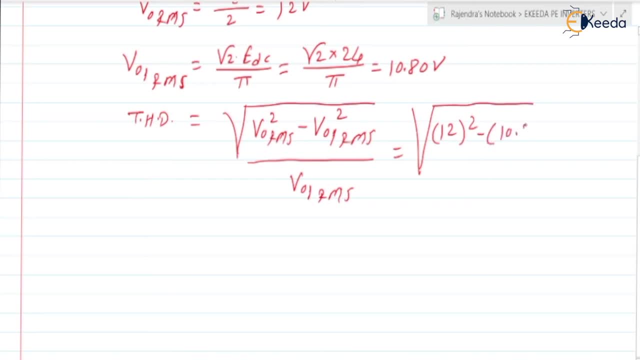 minus 10.80 square right. divided by equal, divided by V01 RMS, It is a 10.80.. Okay, So if you check, it is equal to S12 square minus 10.80.. Okay, So this is 0.0843.. That's number 2.. 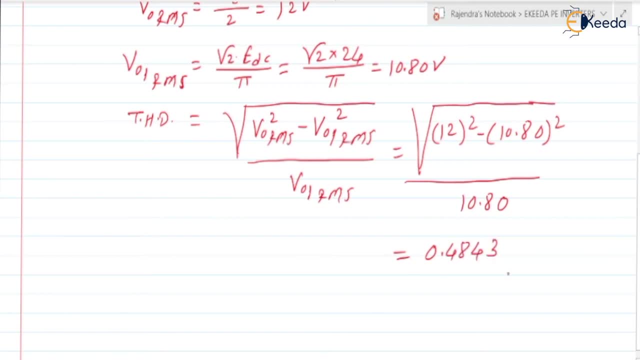 Now we just subtract both. okay, So we subtract the parties from this. okay, So that we just finished everything. Now we sum that, Because this rate is equal to 2 plus SUBSCRIBE point, Okay, it is equal to 3.. 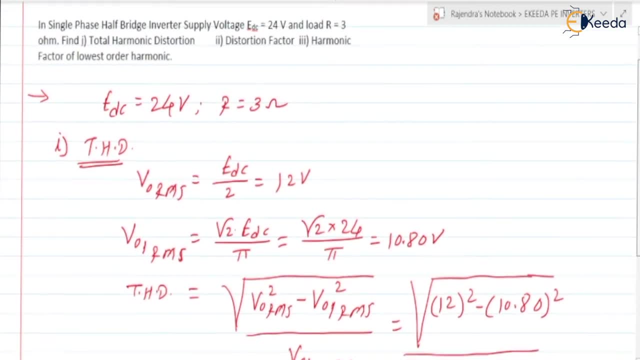 That's 4.. braking the Okay Next. this is about the first bit. In the second bit they ask for the distortion factor. Okay, second bit: The distortion factor DF. Okay, as you may know, the DF is nothing but a ratio of. 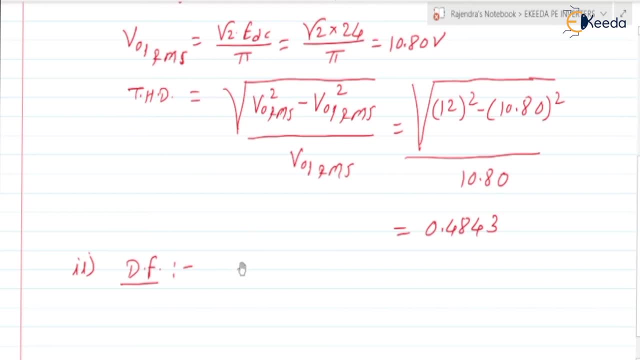 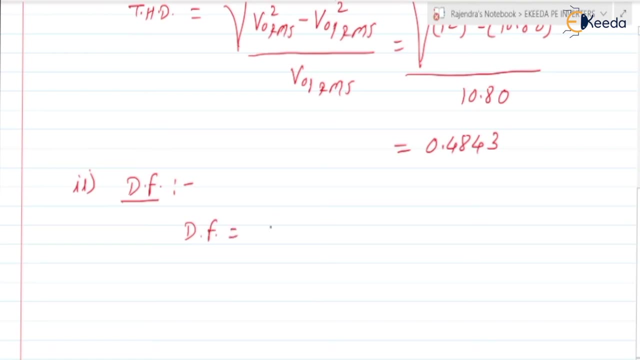 D. There this is zero. certainly most ok, But here, by the end, we want that D nation, falando Ao Après ratio of yes, V0EF is equal to V01RMS divided by V0RMS, right? so what is the V01RMS? it is. 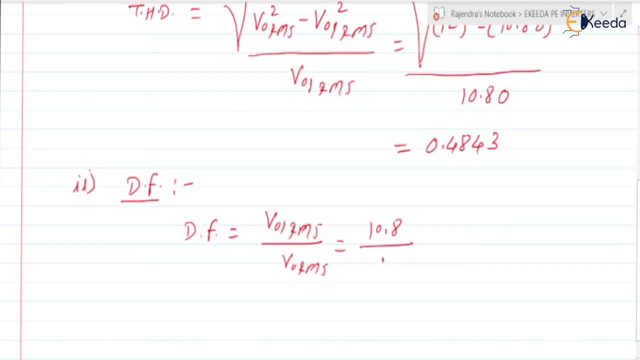 the 10.8 divided by V0RMS is 12, right. so we can find it as 10.8 divided by 12. so it is the 0.9, right, or it is a 90%. we can write okay. similarly the third bit they have asked.